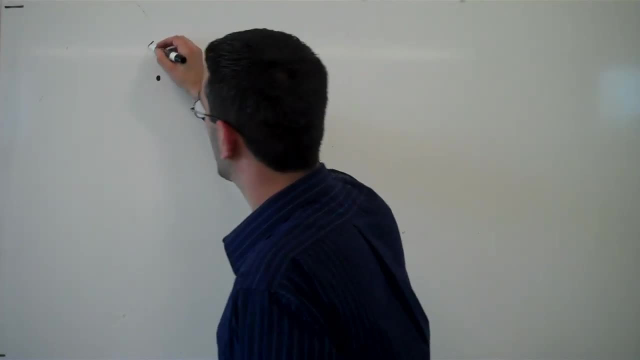 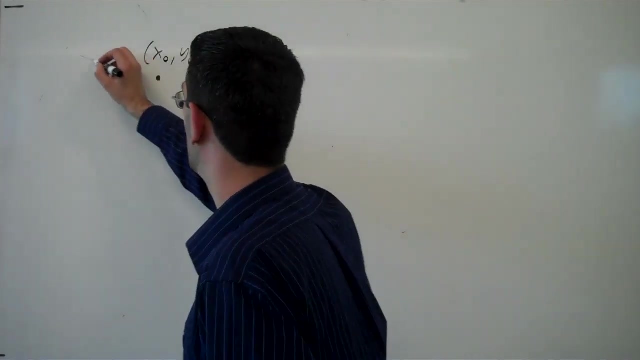 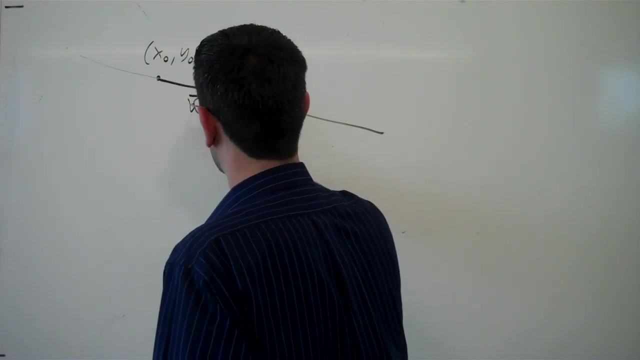 So let's suppose I have a point out here- x-naught, y-naught, z-naught- and I have a direction that my line is going to travel in. So let's imagine I have a vector on this line and we'll call it the vector v. 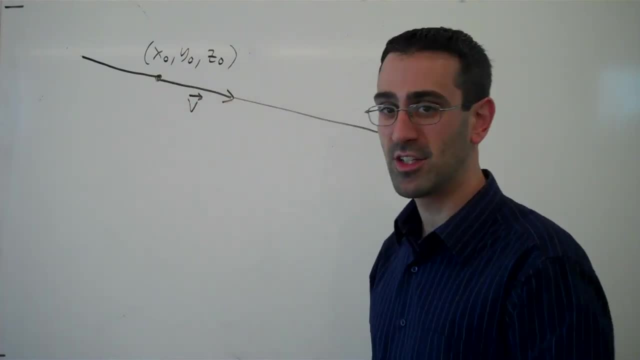 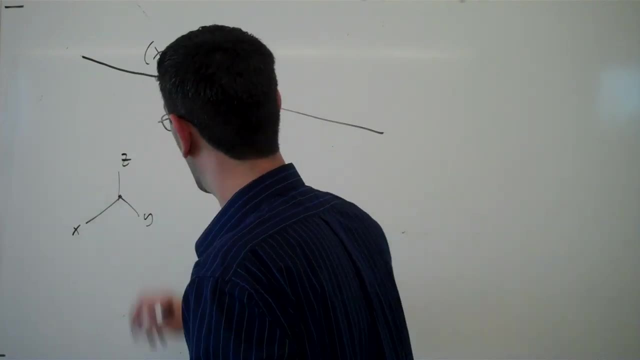 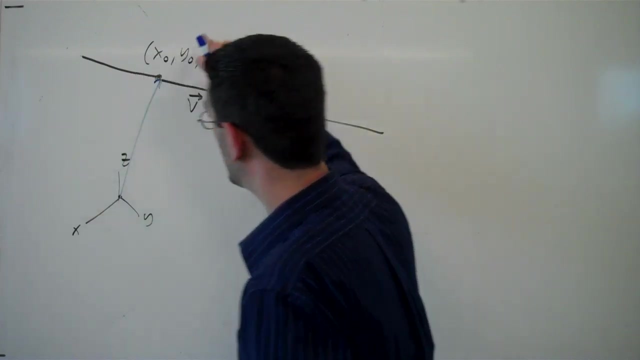 So we've got a point on space, we've got a vector pointing in the direction of the line or parallel to the line, So we're going to introduce- let's imagine that we have the origin down here somewhere- We're going to introduce a position vector, a vector from the origin out to this point, and we'll call it r-naught. 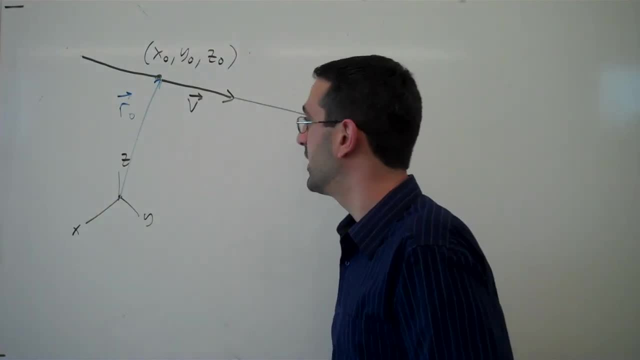 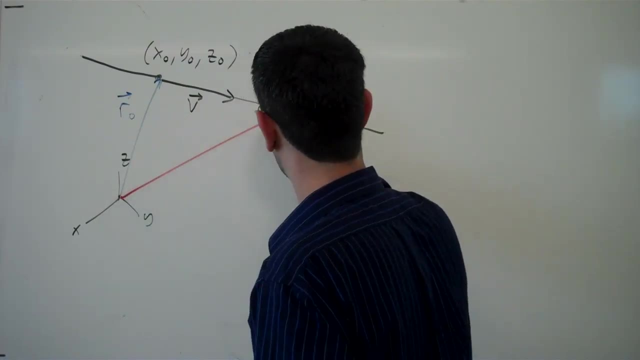 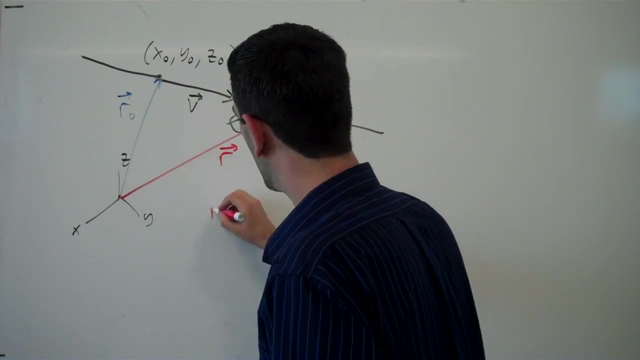 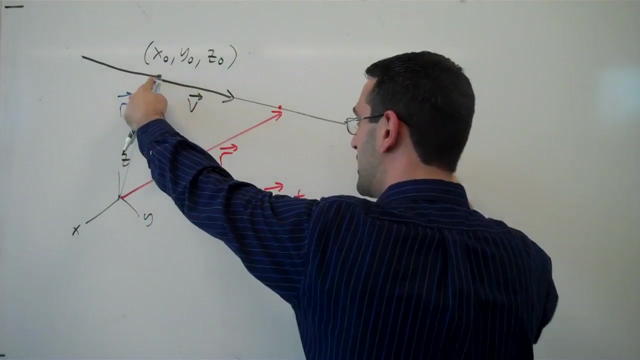 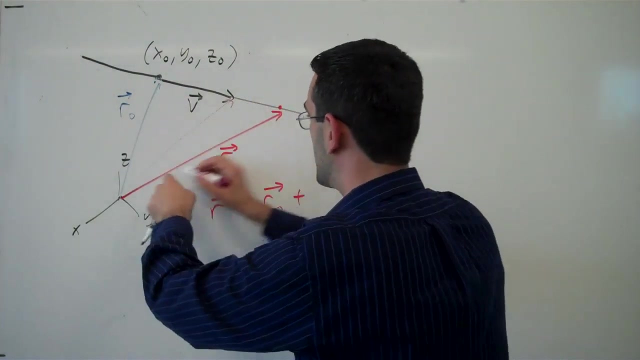 Then any point on the line can be represented as the sort of end of a vector r, where that vector r is the original r-naught point plus some scaling of the vector v right, Because this would be r-naught, This might be r-naught plus 1v, this might be r-naught plus 2v, 3v, 4v, right. 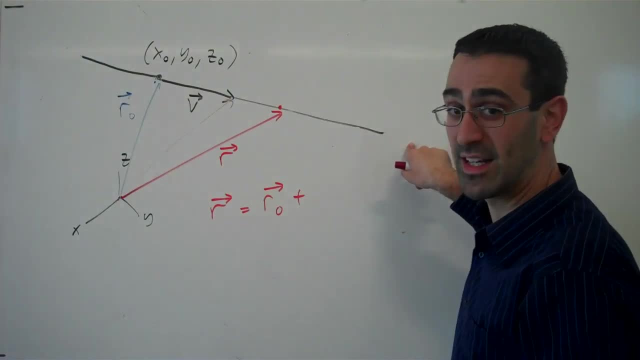 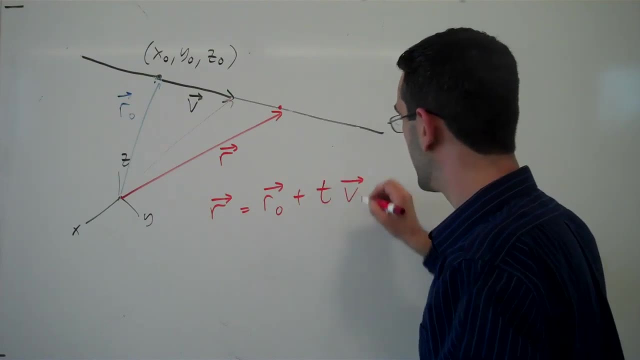 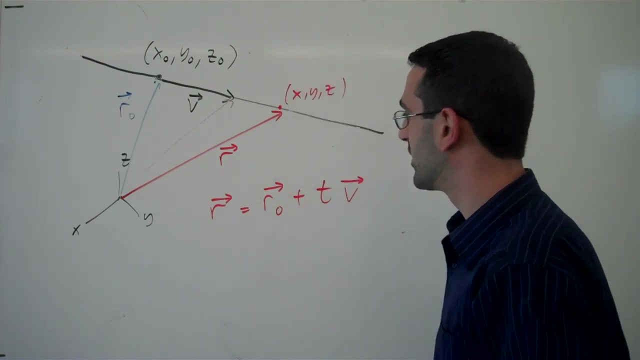 We're combining this vector r-naught with scalings of that vector v, And if we scale that vector v by t, then any vector r pointing to some point, x, y, z on the line can be represented as r-naught plus t times v. 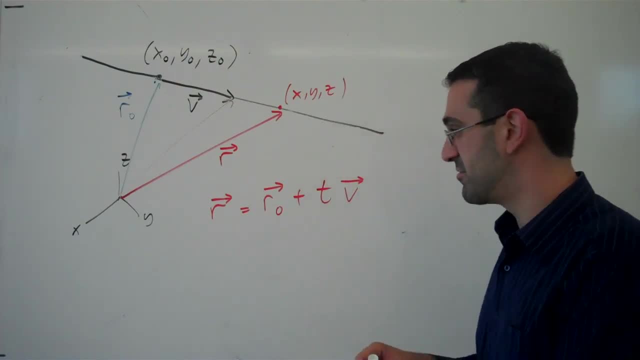 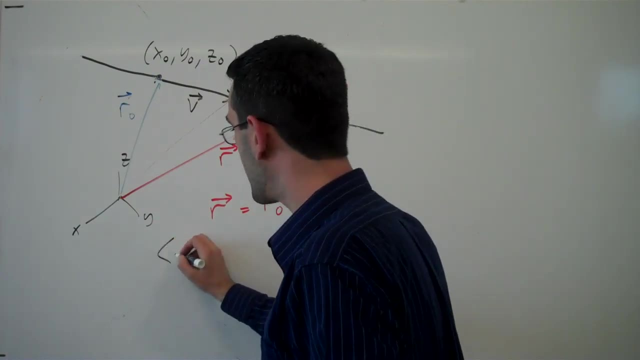 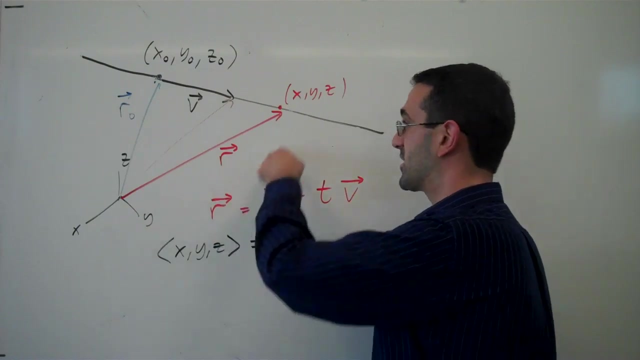 Now, in some cases this vector form of a line is not horribly convenient. so we could break this down and say: the vector v is the vector pointing to x y z. so it is the position vector x y z, right. 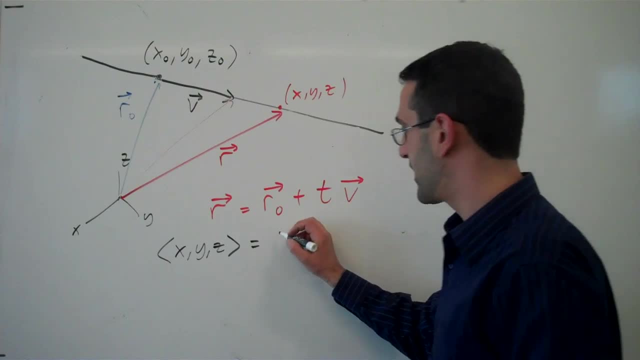 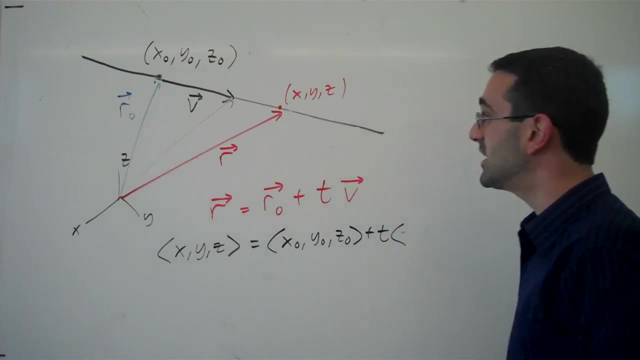 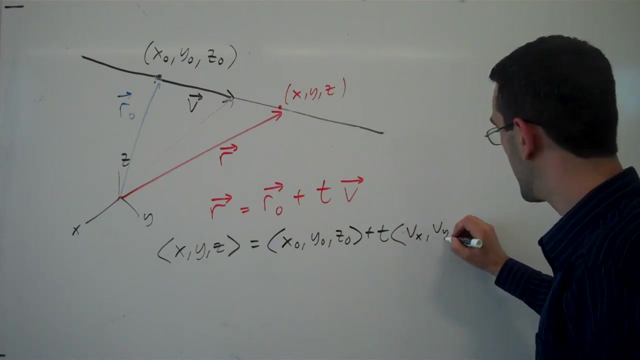 This would be the vector from the origin out to x, y, z. The vector r-naught here is x-naught, y-naught, z-naught. And let's say the vector v has components v-sub-x, v-sub-y and v-sub-z.